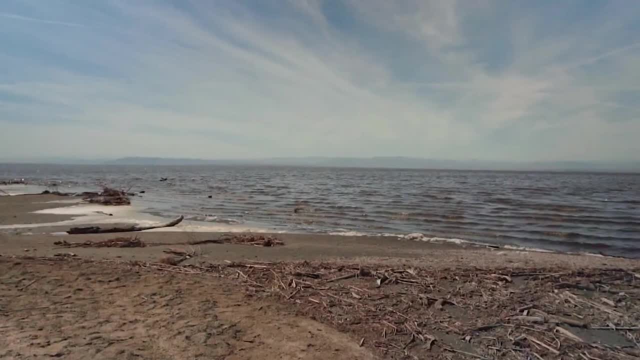 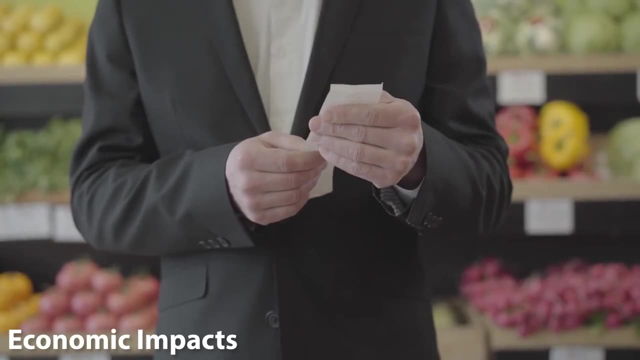 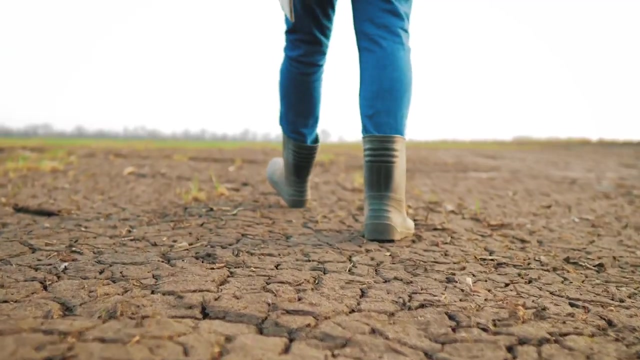 Additionally, our oceans are becoming more acidic, which messes with the marine food chain, especially fish populations. Economic impacts: People's jobs are getting hit hard by climate change. Fields like agriculture, fishing and even tourism are feeling the pinch as nature becomes less predictable. 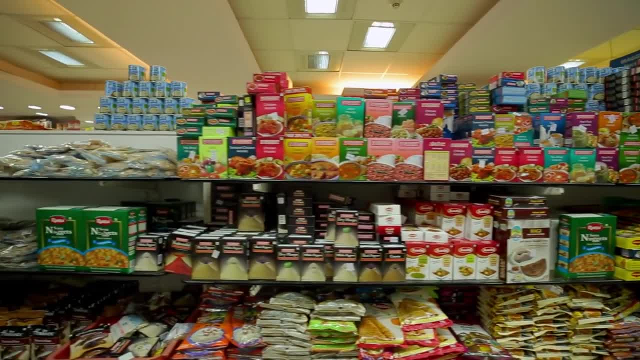 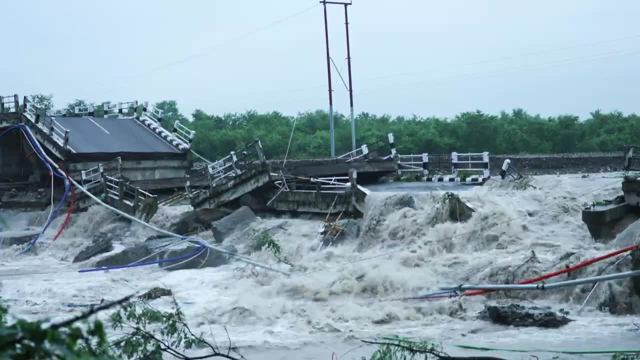 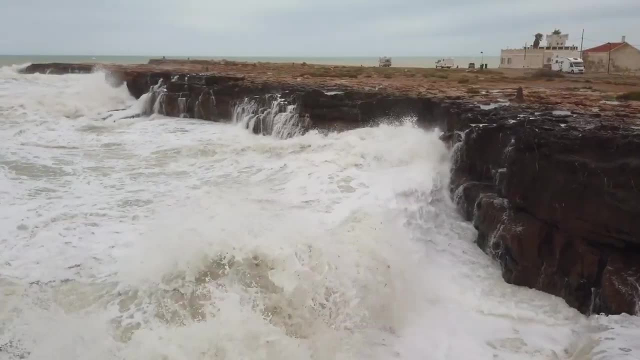 Food prices are going up because there's less produce available, And when extreme weather strikes, the damage to roads, bridges and buildings can cost a tonne to repair. Our beautiful coastlines are under threat. With rising sea levels. beaches are eroding. 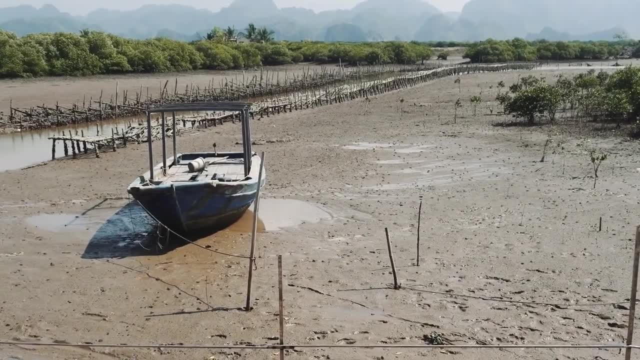 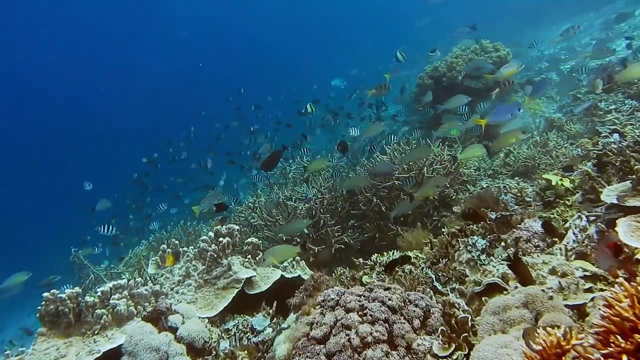 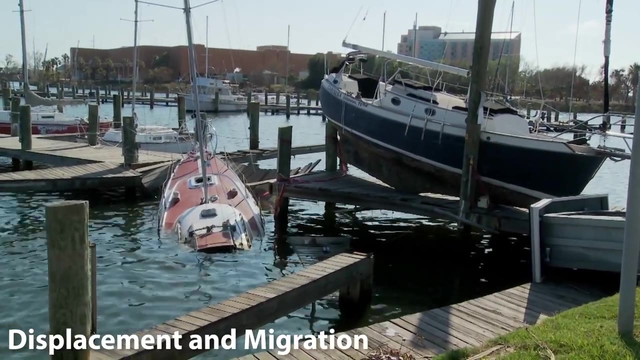 and we're losing vital habitats like the protective mangroves and colourful coral reefs. These aren't just picturesque spots. They play a huge role in supporting diverse marine life and protecting the coast from storm surges, Displacement and migration. Imagine being forced to leave your home. 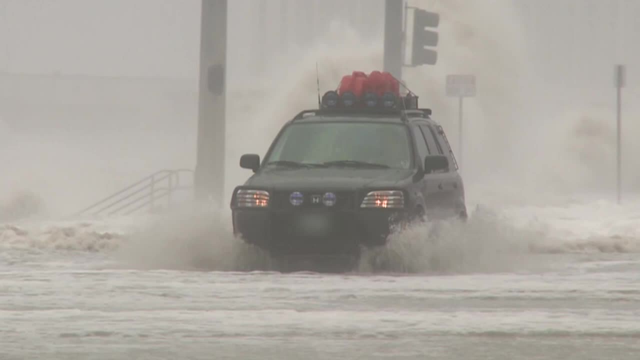 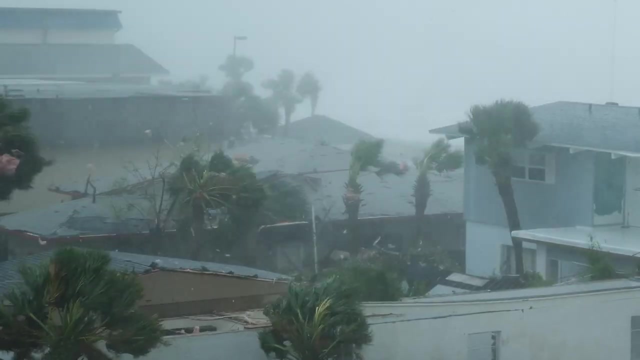 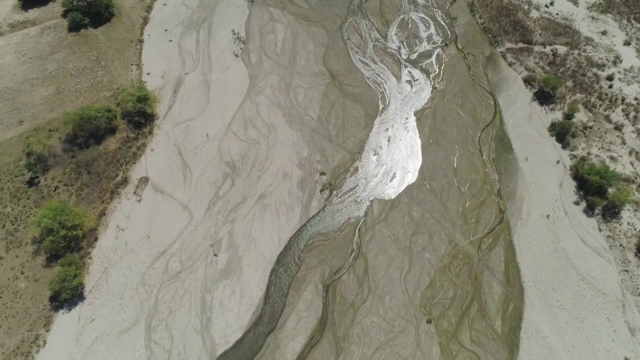 because it's either underwater or too dry to live in. That's the reality for many, as seas rise, following up coastal areas and even entire islands. Meanwhile, violent weather events, from hurricanes to floods, are uprooting entire communities And, in some places, 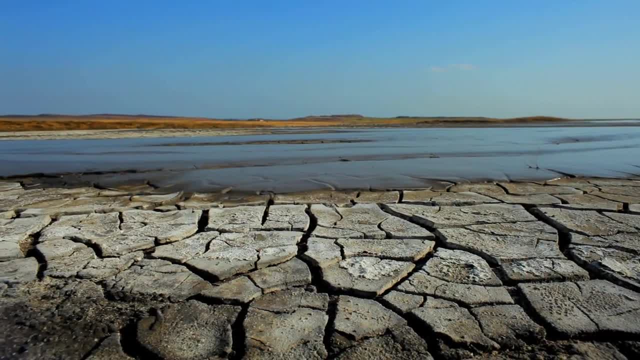 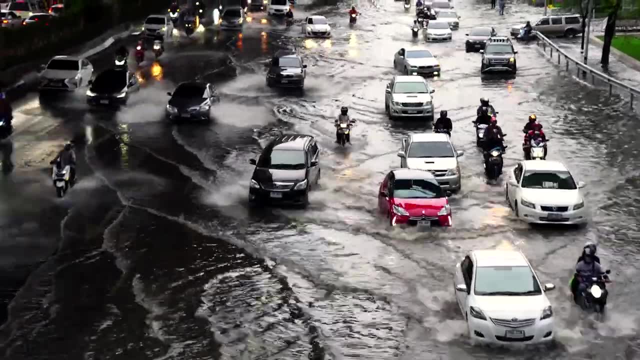 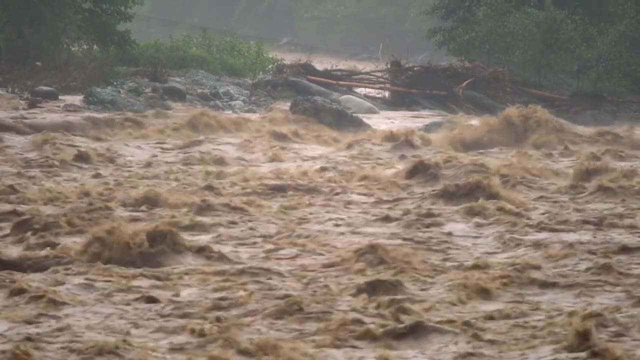 constant droughts and expanding deserts mean people have to move elsewhere to find water and resources to survive As the planet continues to experience these profound changes, the ripple effects touch every corner of our lives. The challenges presented by climate change are not just environmental. 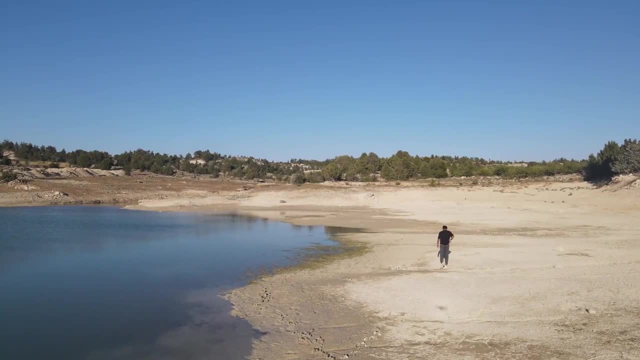 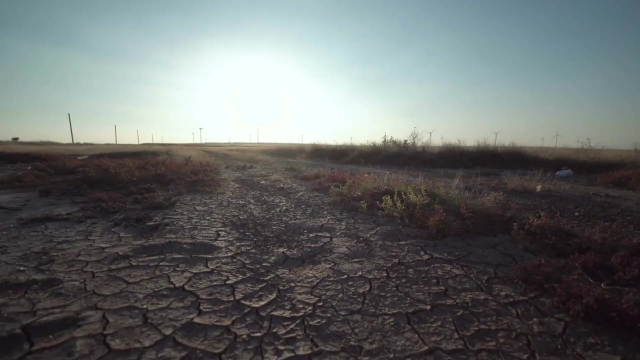 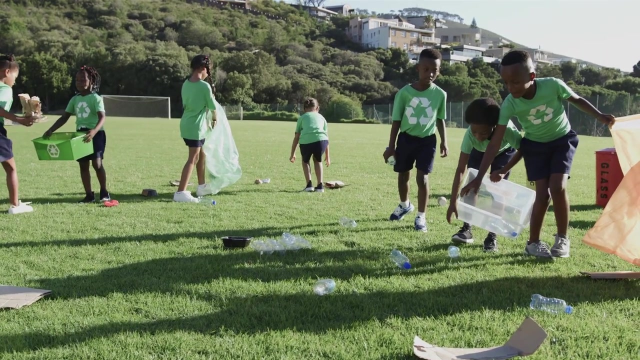 but deeply personal. They affect our health, our food, our livelihoods and even our homes. Yet understanding these impacts gives us the knowledge and the motivation to make a difference. Every effort counts, and by working together and making informed decisions. 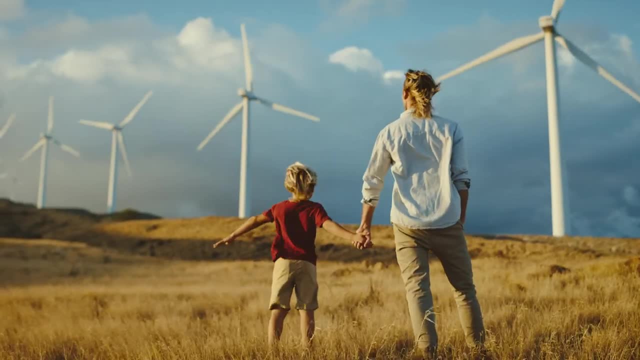 we can pave the way for a more sustainable and hopeful future. Don't forget to subscribe.